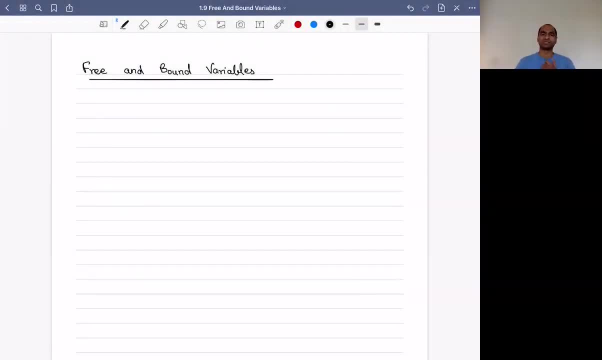 Now I'm going to talk about free and bound variables. They're just two very small definitions, So we'll go quickly. What is a free and bound variable? A variable with a quantifier called bound, Otherwise it's called free. For example, if I just wrote a blanket expression, x plus one is equal to x. 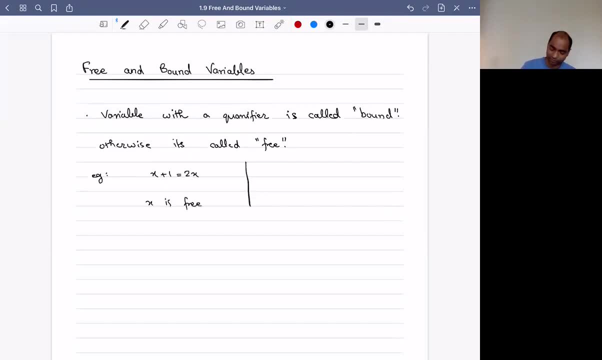 then here x is free. But if I were to write either for x- x plus one is equal to two x, and I also tell you the domain. So here, the domain, let's see, is natural numbers- Or I could have, just I could have used the other quantifier, the existential quantifier. 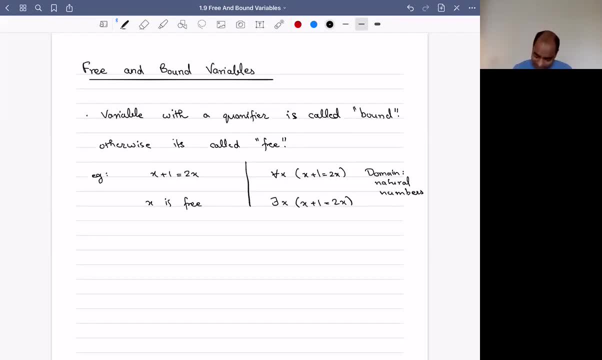 which becomes there exists an x, is that x plus one is two x. Both of these imply that x is bound. Zip is nothing more. It's very simple: If there is a quantifier, it's bound, If there is none, then it's free. 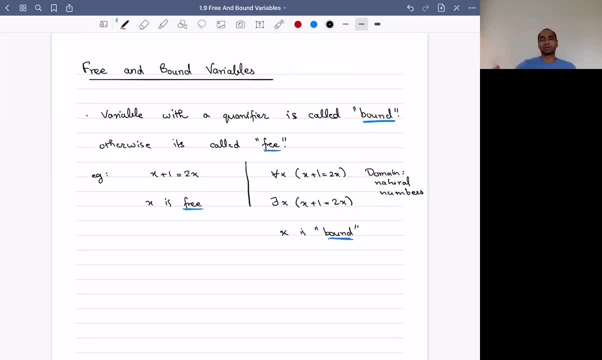 For most of my, or at least like for most of mathematics that you are going to study, you hit abstract algebra and something more complicated, Or even then you don't want free variables. Your statements should only involve bound variables. This is the only thing you should remember from this entire chapter, or this entire concept. 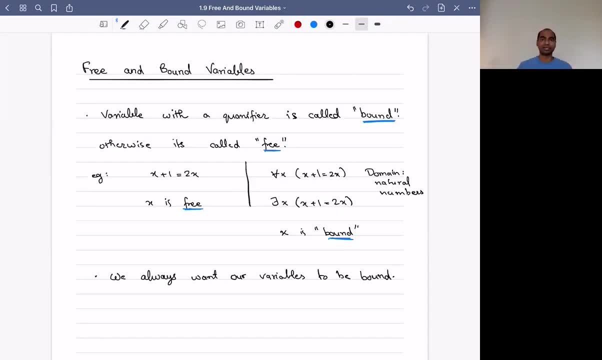 that free is bad, because x plus one equals two. x is not really a proposition. What is the x you're looking for? Is it a natural number? Are you trying to show it for all x? Are you trying to show it for some x? There's not enough information in there. 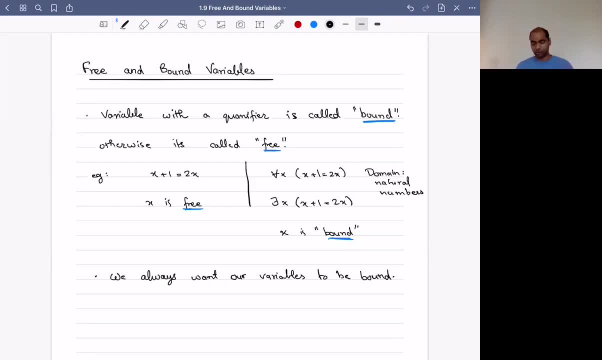 and so it's not considered mathematics. So we always want our variables to be bound. This is easy in logic because you see a variable. it's very easy to say that, oh, there's a missing quantifier. This is much harder when you write proofs in English.